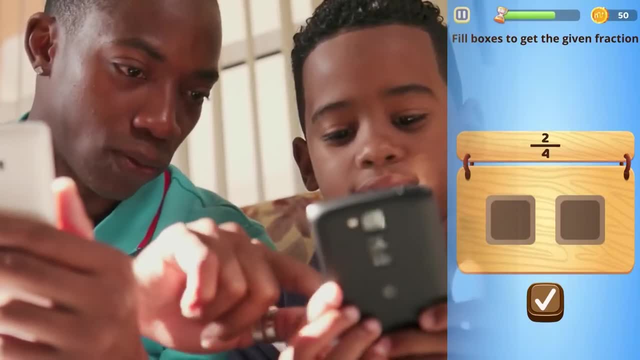 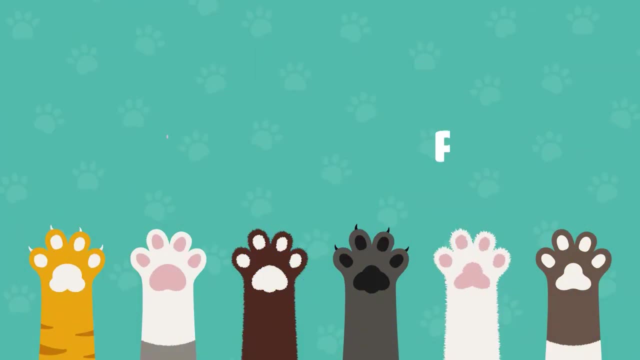 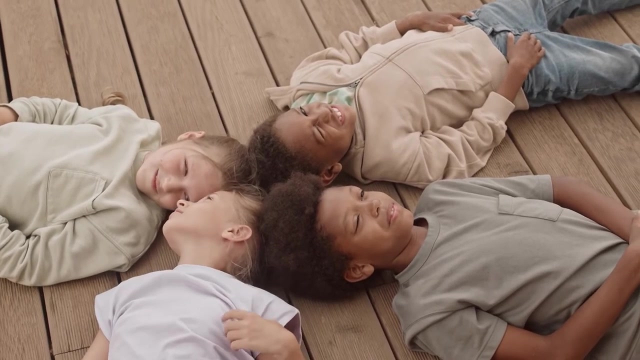 determine which strengths and abilities they can improve, boost their academic performance and exercise their minds and bodies with Mental Up. one app for all. President's Cat. This game is an excellent exercise for kids' vocabulary and attention skills. All they need to do is find adjectives. 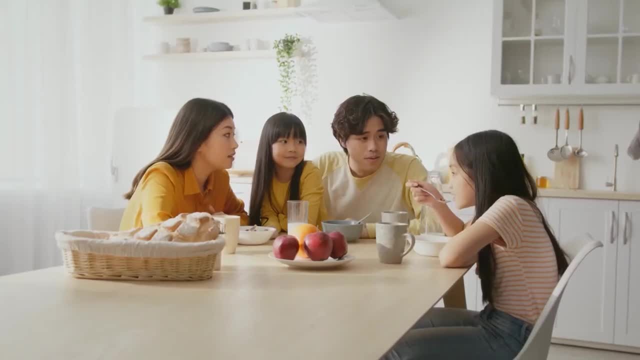 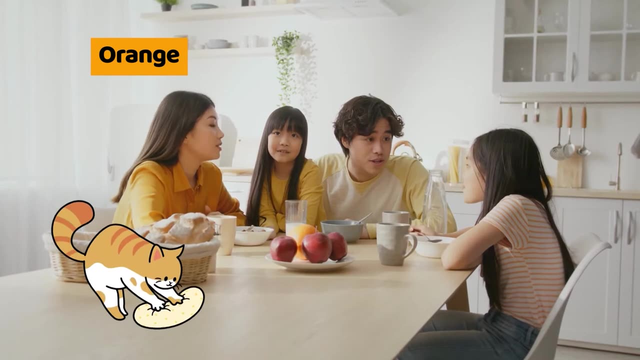 to describe the president's cat, For example, the first player can start with: The president's cat has orange fur. After saying the first adjective, the second player should describe the cat with another one, such as: The president's cat has orange and soft fur. 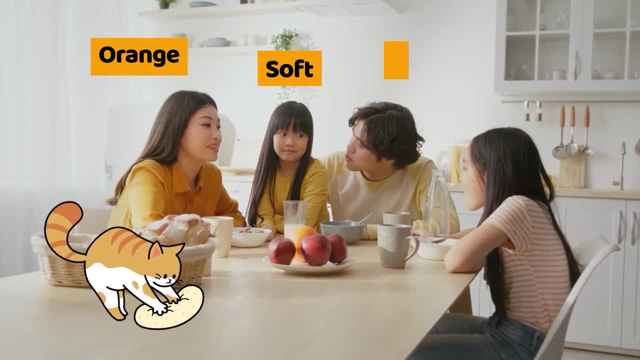 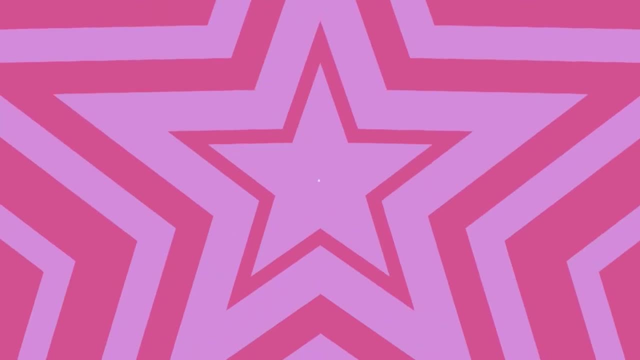 The third player can say: The president's cat has orange, soft and long fur, and so on. The game continues until one kid forgets the adjective's order or can't find a new one. Find the Location. Here's a great indoor activity for 7-8-year-olds. 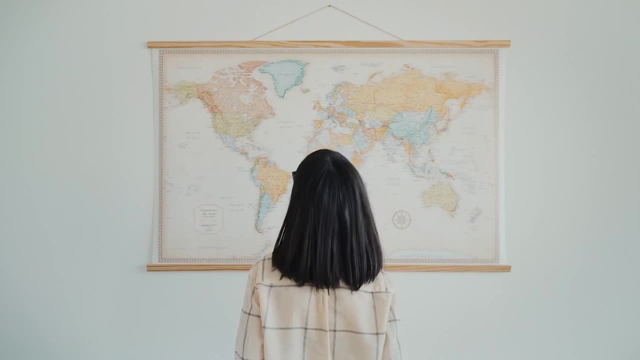 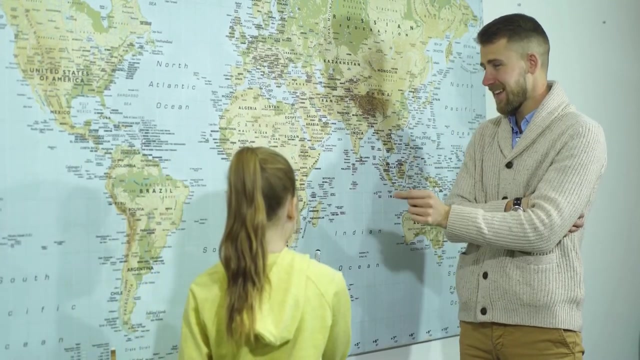 Hang a map on the wall and randomly say a country, mountain or stream name, then ask the children to show it on the map. The first kid who finds it wins a point. With this game they can improve their attention skills as well as geographical knowledge. 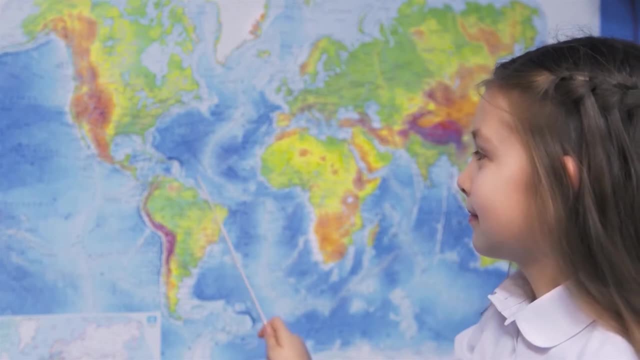 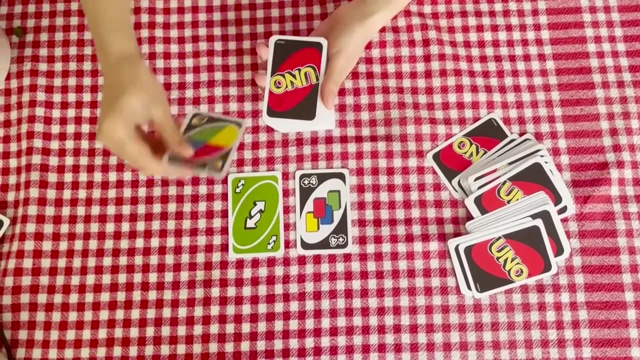 Let's talk next about one of the best card games for children of all ages: Uno. Uno cards have both numbers and colors, with some unexpected rules like skipping and reversing the order of card play from time to time, Even if the rules are easy to understand. 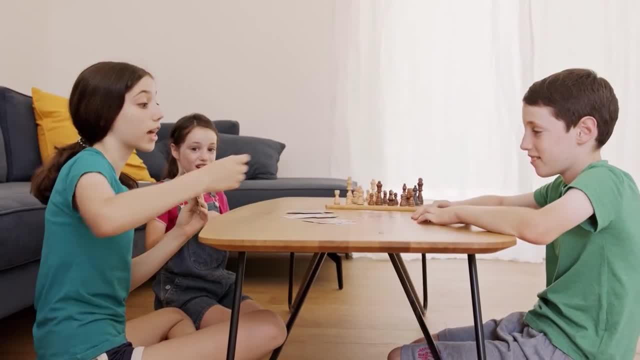 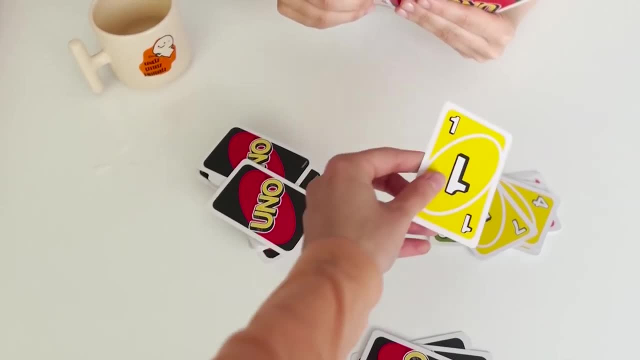 it still improves strategic thinking, memory, attention and social skills. You can't even imagine a deck of Uno cards could cause that much laughter, So it's a great time to pick one of them up and play. Your kids can discover MentalUp's. 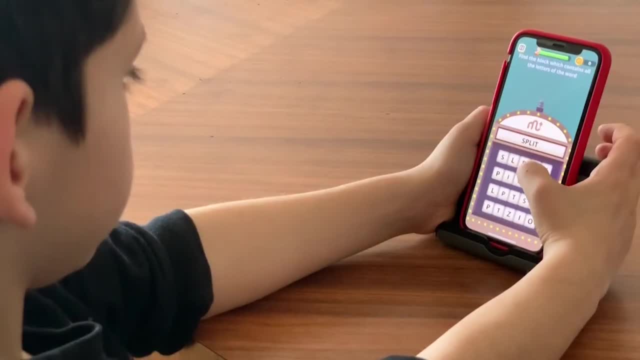 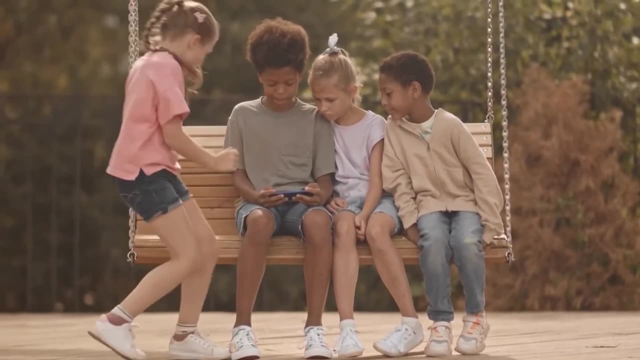 hundreds of games even now. No need to wait for their friends to do entertaining activities. Download MentalUp and start your kid's development journey. You can keep reading other suggestions for our other learning games by clicking the link in the description box. By the way, if you want to learn more about MentalUp, check out the link in the 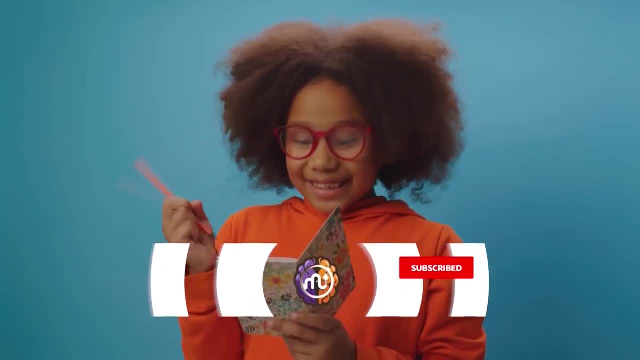 description box. If you want to learn more about MentalUp, click the link in the description box. By the way, if you want to learn more about MentalUp, click the link in the description box. Do you have any ideas for the fifth suggestion? 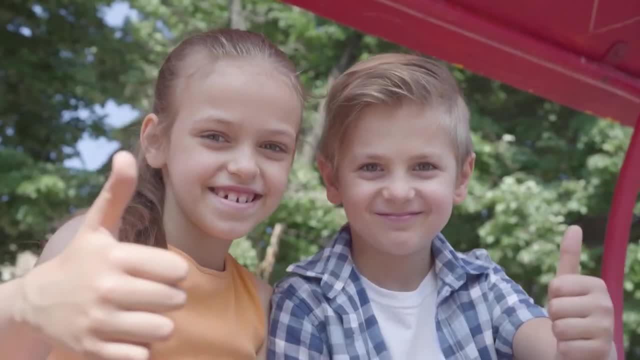 Give us a big thumbs up and meet us in the comments. We can't wait to hear your thoughts.